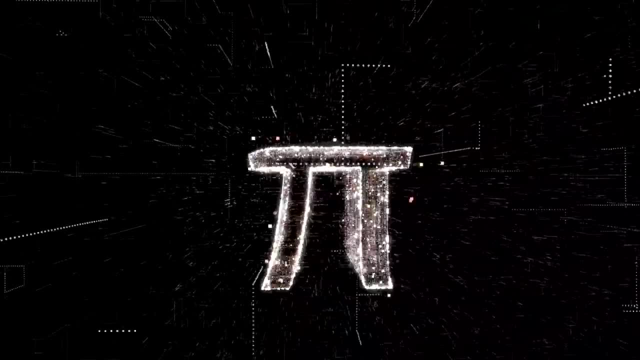 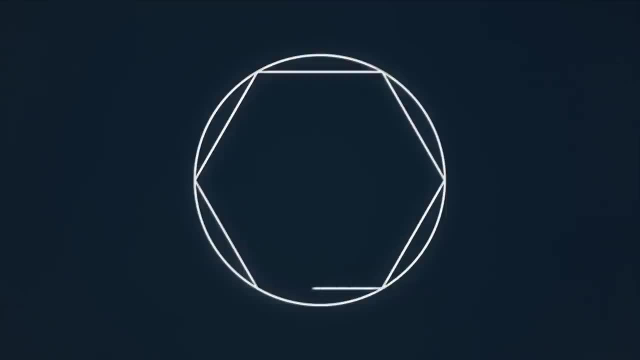 Well, it's sort of the most obvious way. It's easy to show that pi must be between 3 and 4.. Take a circle and draw a hexagon inside it with sides of length 1. A regular hexagon can be divided into six equilateral triangles. 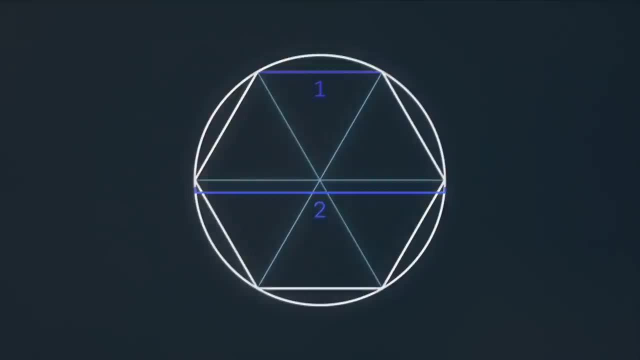 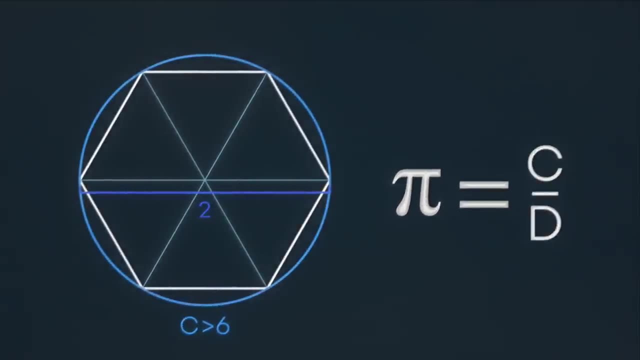 So the diameter of the circle is 2.. Now the perimeter of the hexagon is 6, and the circumference of the circle must be larger than this, so pi is 2.. Pi must be greater than 6 over 2,, so pi is greater than 3.. 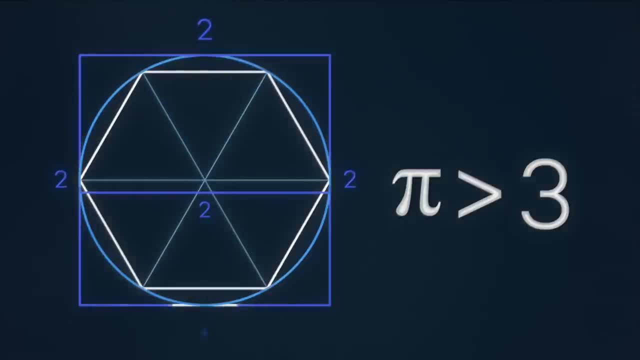 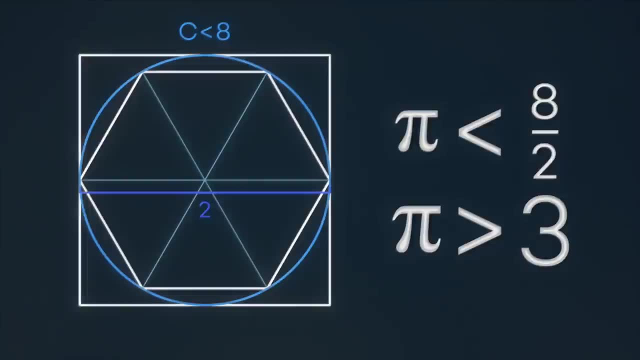 Now draw a square around the circle. The perimeter of the square is 8,, which is bigger than the circle's circumference, so pi must be less than 8 over 2, so pi is less than 4.. This was actually known for thousands of years. 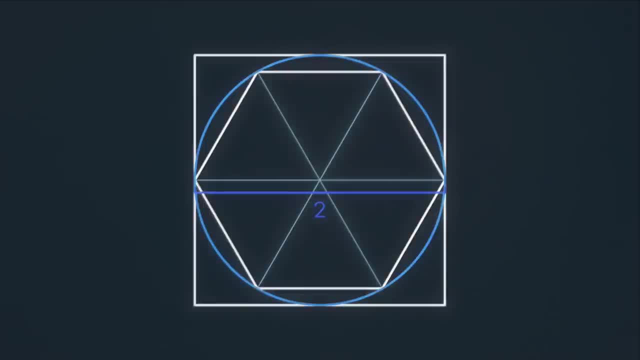 And then, in 250 BC, Archimedes improved on the method. So first he starts with the hexagon, just like you did, And then he bisects the hexagon to a dodecagon. So that's a 12-sided, regular, 12-sided shape. 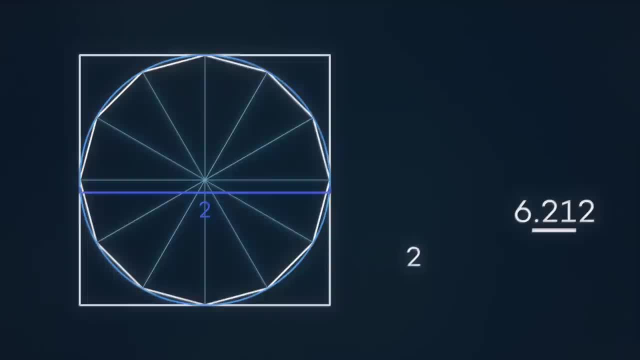 And he calculates its perimeter. The ratio of that perimeter to the diameter will be less than pi. He does the same thing for a circumscribed 12-gon and finds an upper bound for pi. The calculations now become a lot more tricky because he has to extract square roots. 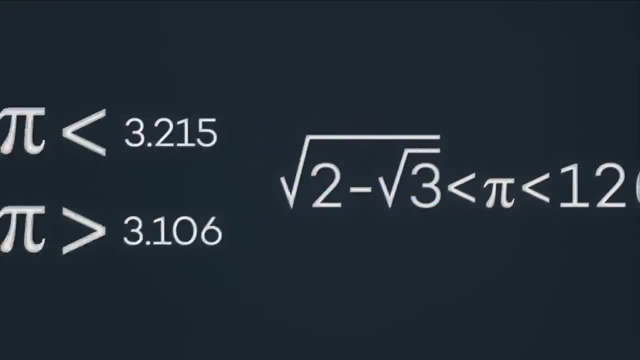 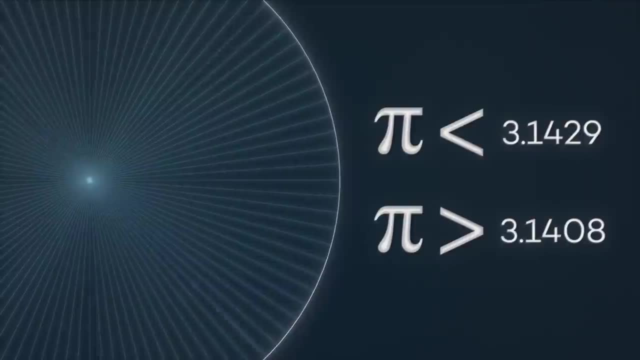 and square roots of square roots and turn all these into fractions. But he works out the 12-gon and then the 24-gon, 48-gon, and by the time he gets to the 96-gon he's sort of had enough. 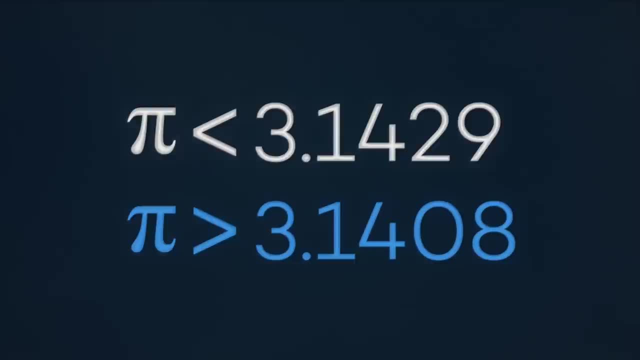 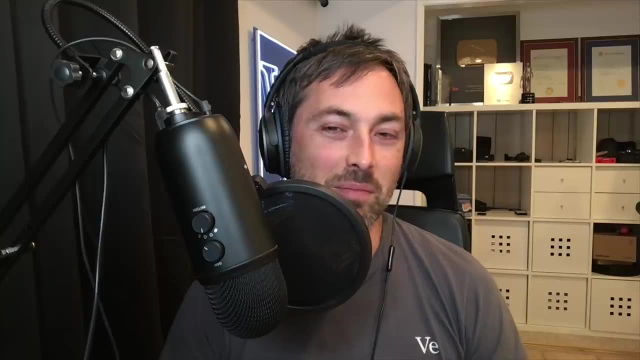 But he gets in the end. he gets pi to between 3.1408 and 3.1429.. So for over 2,000 years ago that's not too bad. Yeah, that seems like all the precision you'd need in pi. 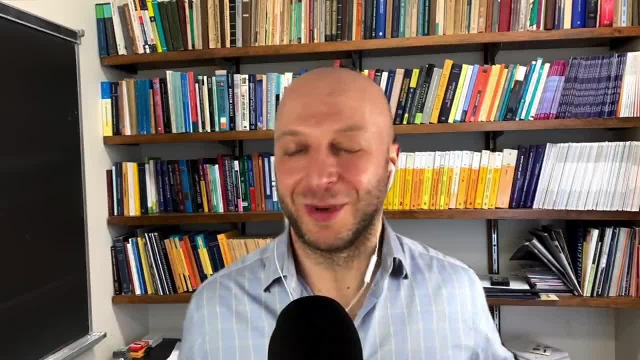 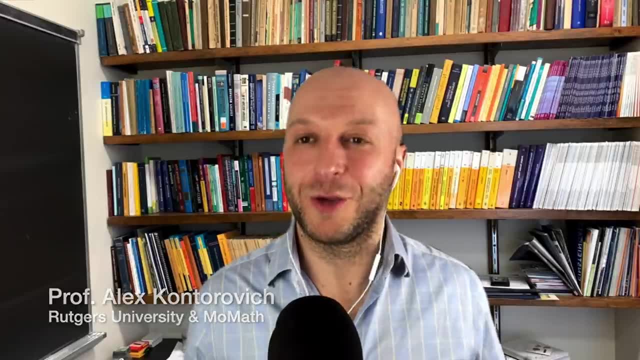 Right. so this goes way beyond precision for any practical purpose. This is now a matter of flexing your muscles. You know this is showing off just how much mathematical power you have, that you can work out a constant like pi to very high precision. 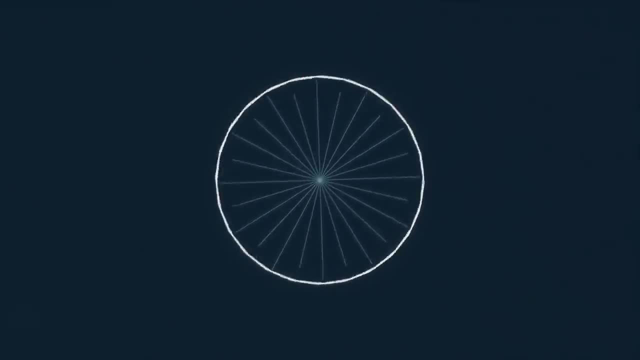 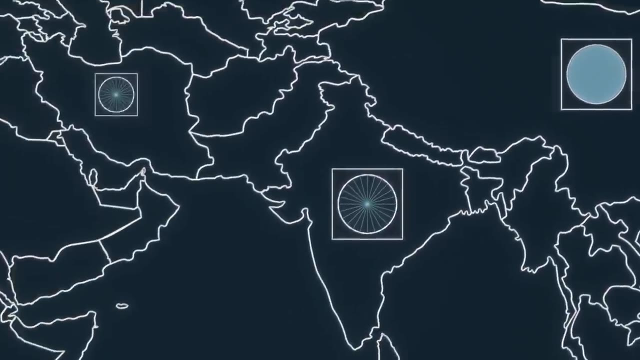 So for the next 2,000 years. this is how everyone carried on bisecting polygons to dizzying heights As pi passed through. Chinese, Indian, Persian and Arab mathematicians each contributed to these bounds along Archimedes' line. 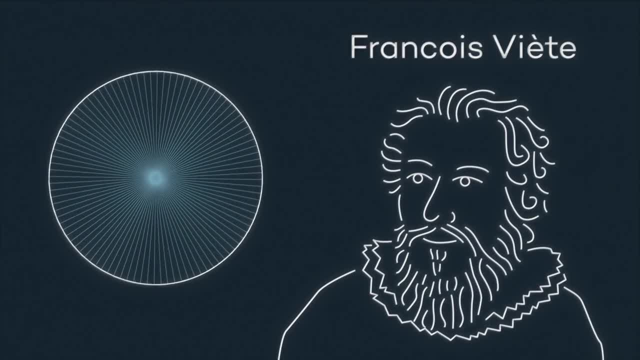 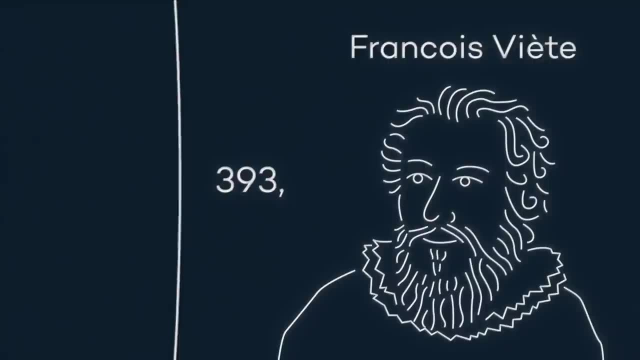 And in the late 16th century, Frenchman François Viette doubled a dozen more times than Archimedes, computing the perimeter of a polygon with 393,216 sides, Only to be outdone at the turn of the 17th century by the Dutch. 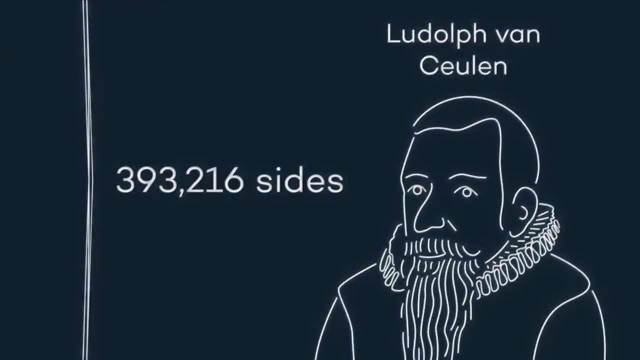 Ludolf van Koeulen. He spent 25 years on the effort computing to high accuracy the perimeter of a polygon with 2 to the 62 sides, That is, 4 quintillion, 611 quadrillion, 686 trillion. 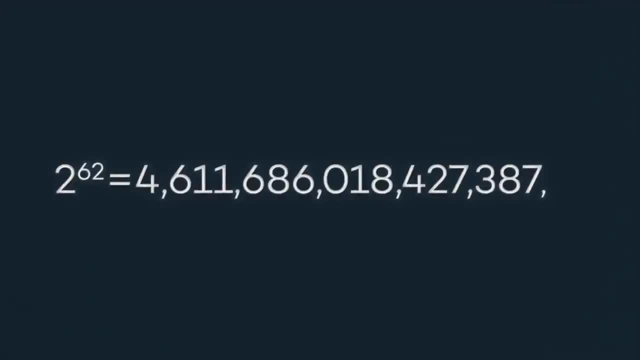 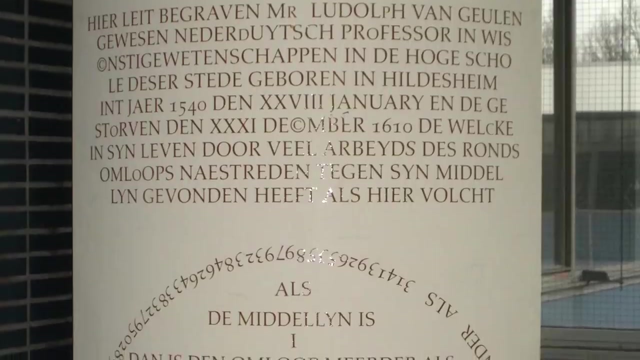 18 billion 427 million 387 thousand 940 billion 4 sides. What was the reward for all of that hard work? Just 35 correct decimal places of pi. He had these digits inscribed on his tombstone. 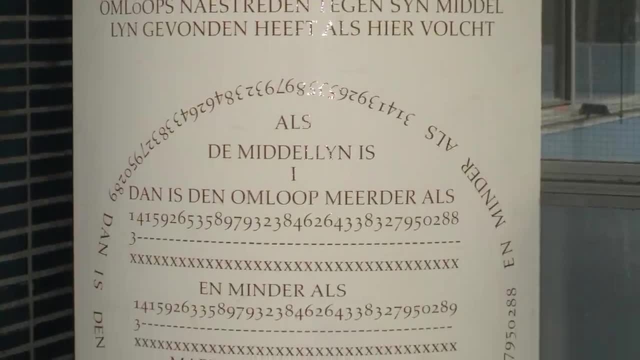 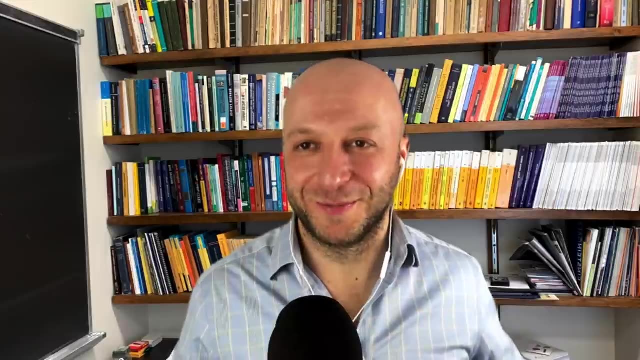 20 years later, his record was surpassed by Christoph Grienberger, who got 38 correct decimal places, But he was the last to do it like this. Pretty much, yeah, Because shortly thereafter we get Sir Isaac Newton on the scene. And uh, once Newton introduces his method, nobody is bisecting Engans ever again. The year was 1666, and Newton was just 23 years old. He was quarantining at home due to an outbreak of bubonic plague. 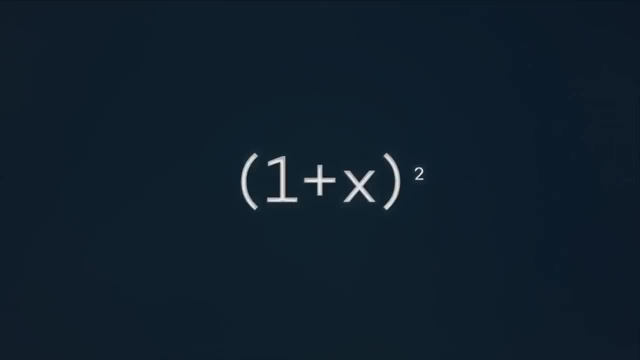 Newton was playing around with simple expressions like 1 plus x all squared. You can multiply it out and get 1 plus 2x plus x squared. Or what about 1 plus x all cubed? Well, again, you can multiply out all the terms and get. 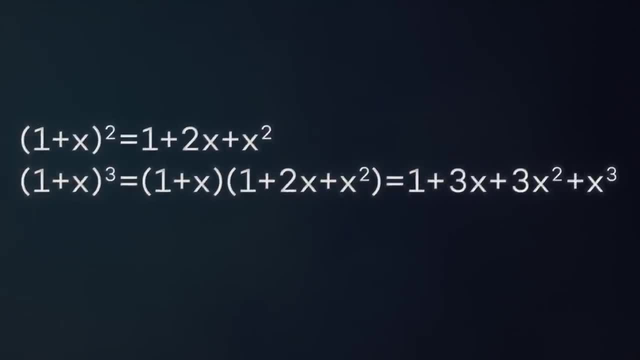 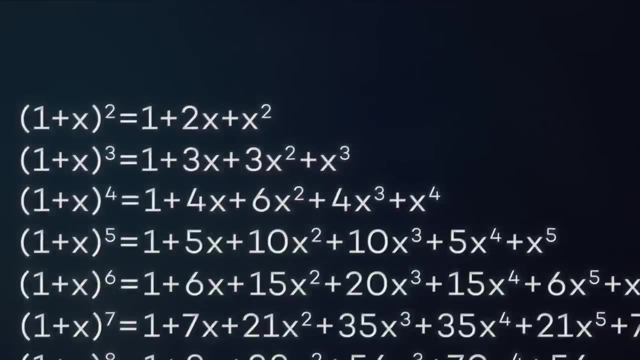 1 plus 3x plus 3x squared plus x cubed, And you could do the same for 1 plus x to the 4, or 1 plus x to the 5, and so on. But Newton knew there was a pattern that allowed him to skip. 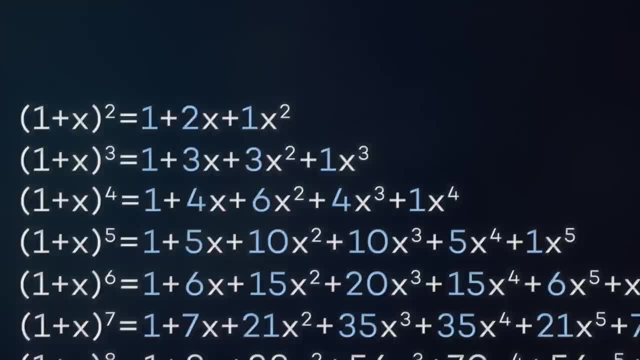 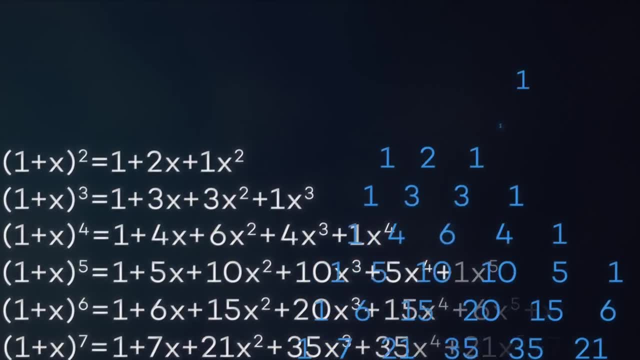 all the tedious arithmetic and go straight to the answer. If you look at the numbers in these equations- the coefficients on x and x squared and so on- well they're actually just the numbers in Pascal's triangle, The power that 1 plus x was raised to. 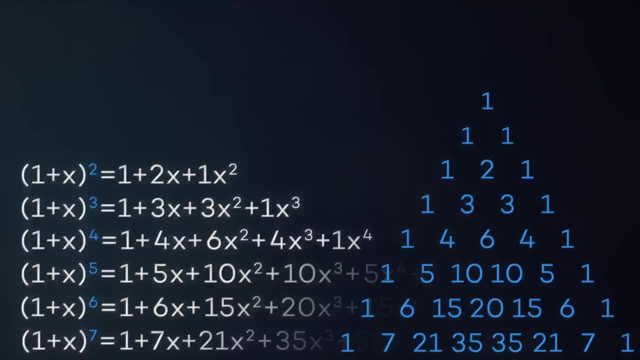 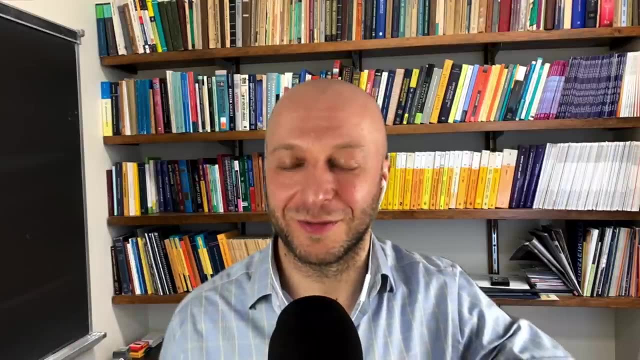 corresponds to the row of the triangle Right, and Pascal's triangle is really easy to make. It's something that's been known from ancient Greeks and Indians and Chinese, Persians. a lot of different cultures discovered this. All you do is, whenever you have a row. 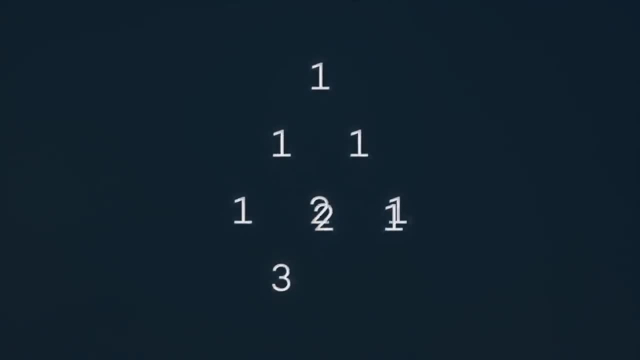 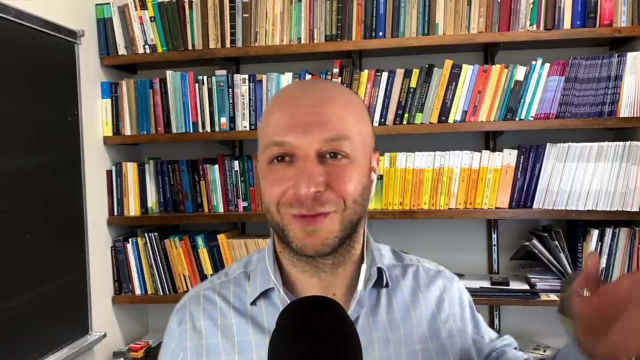 you just add the two neighbors and that gives you the value of the row below it. So that's a really quick, easy thing. You can compute, you know, the coefficients for 1 plus x to the 10 in a second. 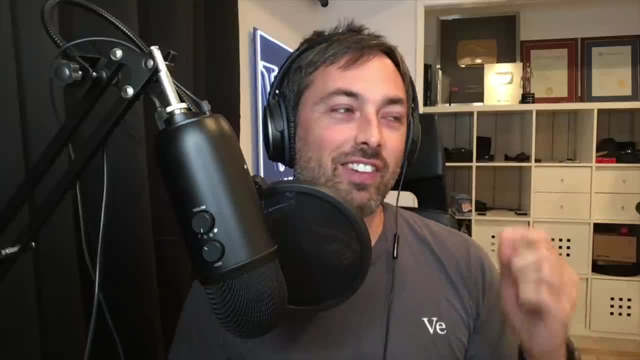 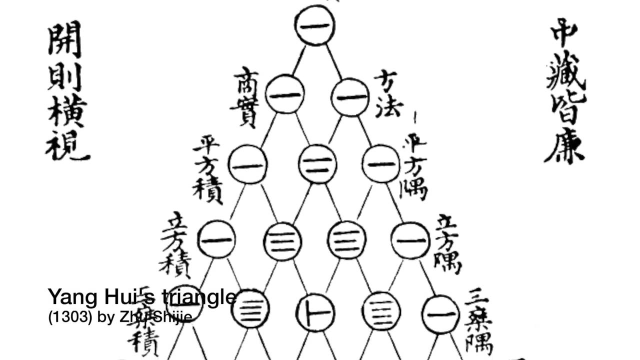 instead of sitting there doing all the algebra. The thing that fascinates me when I started looking at those old documents was how, even like I don't speak those languages, I don't know those number systems, and yet it is obvious, it is clear as day. 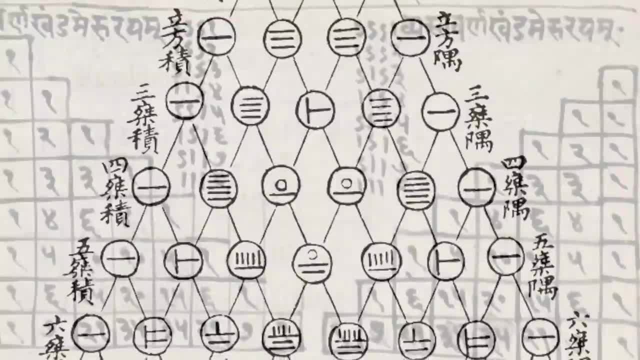 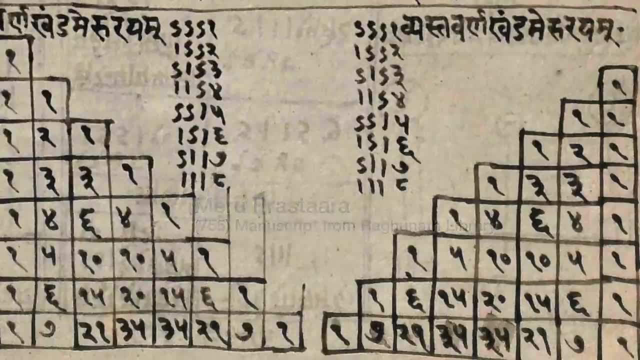 that they are all writing down the same thing, which today, in the Western world, we call Pascal's triangle. That's the beauty of mathematics: It transcends culture, it transcends time, it transcends humanity. It's going to be around well after we're gone. 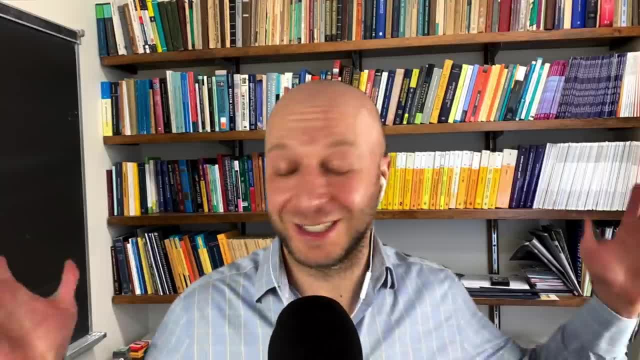 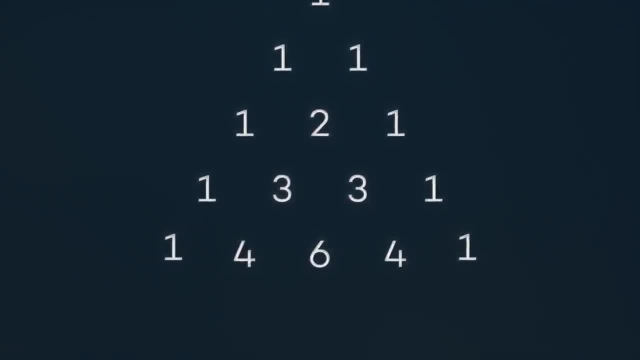 and ancient civilizations. alien civilizations will know Pascal's triangle. Over time people worked out a general formula for the numbers in Pascal's triangle, So you can calculate the numbers in any row without having to calculate all the rows before it. For any expression, 1 plus x to the n. 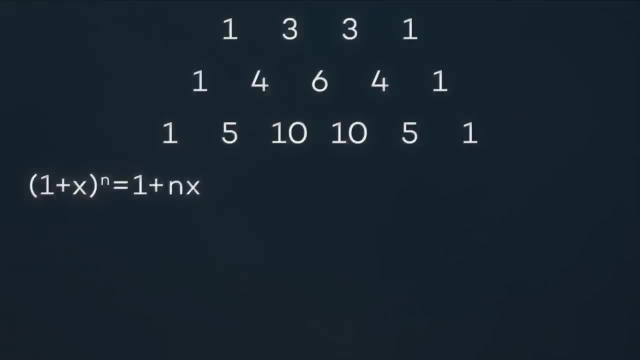 it is equal to 1 plus n times x plus n times n minus 1 x, squared on 2 factorial plus n times n minus 1 times n minus 2 times x, cubed on 3 factorial and so on, And that's the binomial theorem. 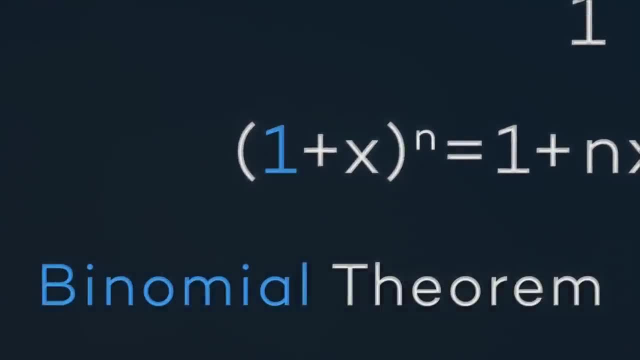 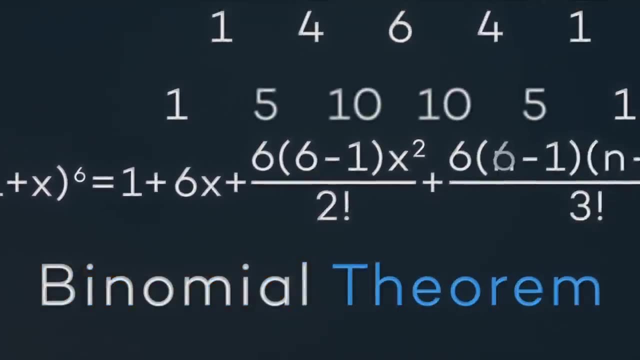 So binomial, because there's only two terms, 1 and x. bi is 2, there's two nomials, And theorem is that this is a theorem that you can rigorously prove that this formula is exactly what you'll see. 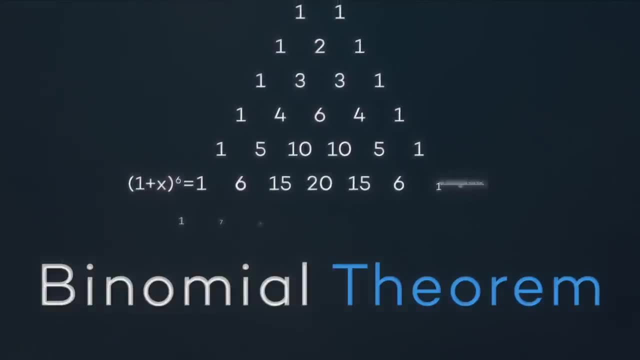 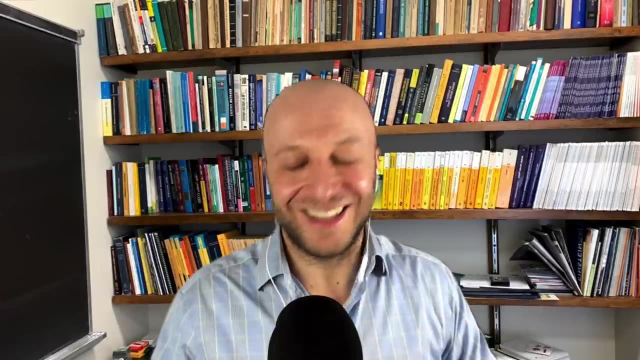 as the coefficients in Pascal's triangle. So all of this was known in Newton's day already. Yeah, exactly, Everybody knew this. everybody saw this formula and yet nobody thought to do with it. the thing that Newton did with it, which is to break the formula. 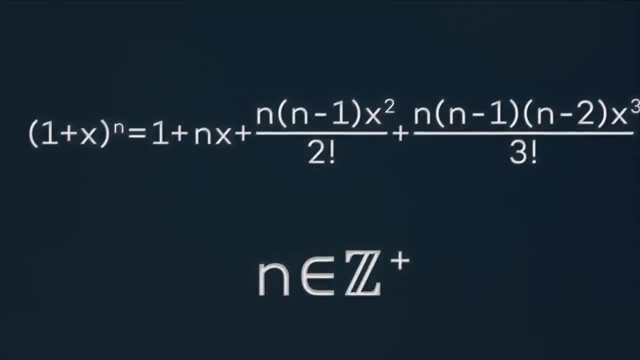 So the binomial theorem insists that you apply it only when n is a positive integer, which makes sense, right? This whole thing is about working out 1 plus x times itself a certain number of times. But Newton says: screw that, just apply the theorem. 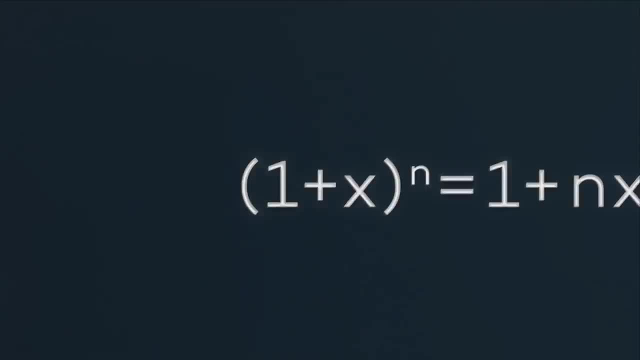 I mean, math is about finding patterns and then extending them and trying to find out where they break. So he tries 1 plus x to the negative 1.. So that's 1 over 1 plus x. What happens if I just blindly plug in? 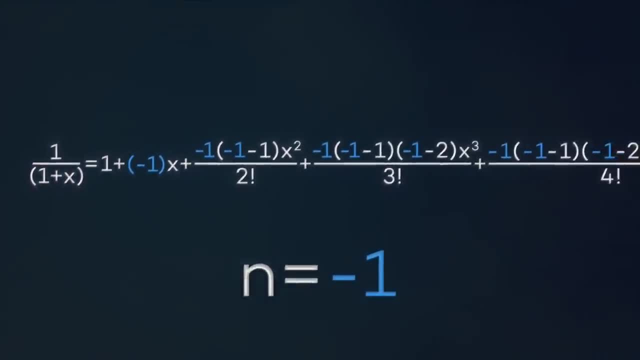 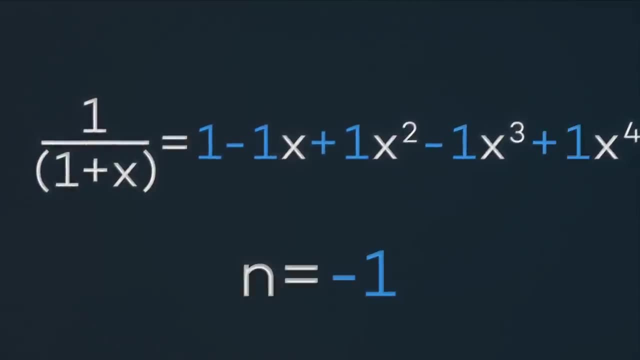 n equals negative 1 for the right-hand side of the formula, And what you get is the terms alternate back and forth: Plus 1, minus 1, plus 1, minus 1, and so on forever. So that's 1 minus x. 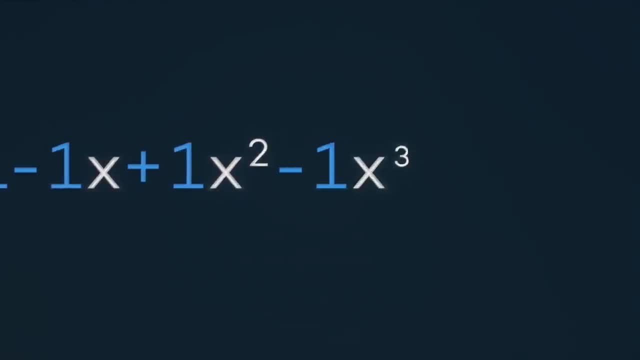 The next term will be a plus x squared. The next term will be a minus x cubed. plus x to the fourth, minus x to the fifth. So it's just alternating series with plus and minus signs as the coefficients, So it becomes an infinite series. 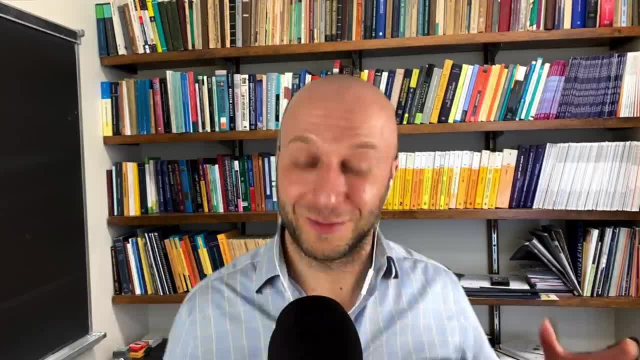 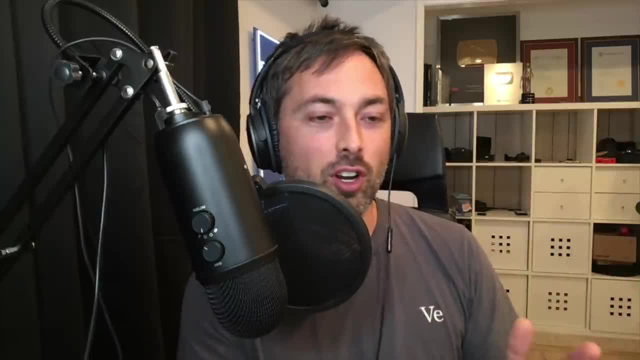 Yeah, that's right. If you don't have a positive integer, the binomial theorem- Newton's binomial theorem- will give you an infinite sum. But how do you understand that? Like for all positive integers, it was just a finite set of terms. 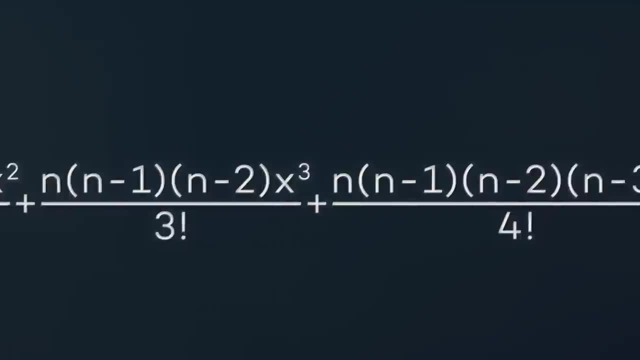 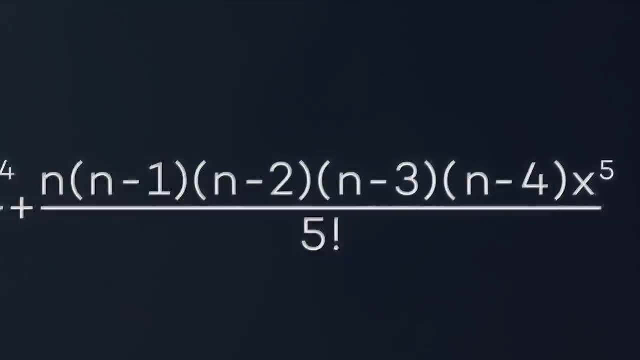 and now we've got an infinite set of terms. Yeah, so what happens is, if you have a positive integer- you remember that formula- the coefficient looks like n times n minus 1, times n minus 2, and so on. When you get to n minus n, 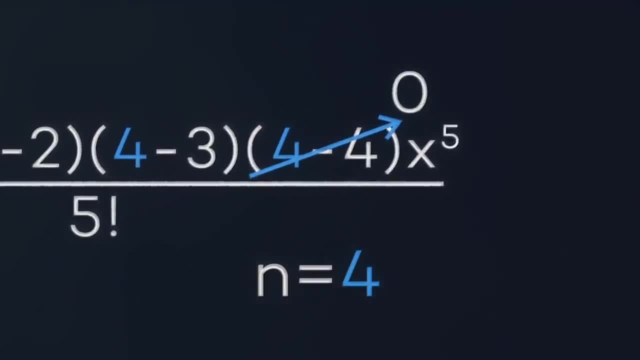 if n is a positive integer, you will eventually get there. and n minus n is 0.. So that coefficient and all the coefficients after it are all 0, and that's why it's just a finite sum, It's a finite triangle. 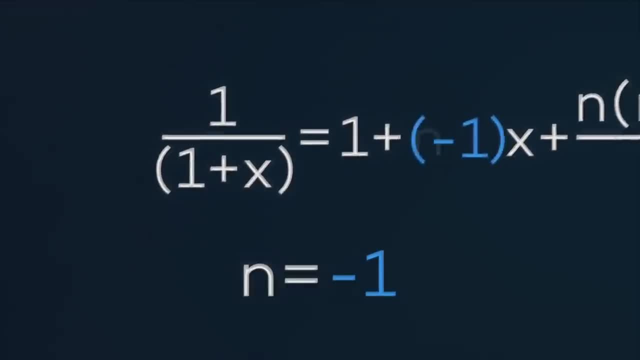 But once you get outside of that the triangle with positive integers, you never hit n minus n, because n is not a positive integer. So you get this infinite series. So I think the big question is: does this actually work? Does Newton's infinite series? 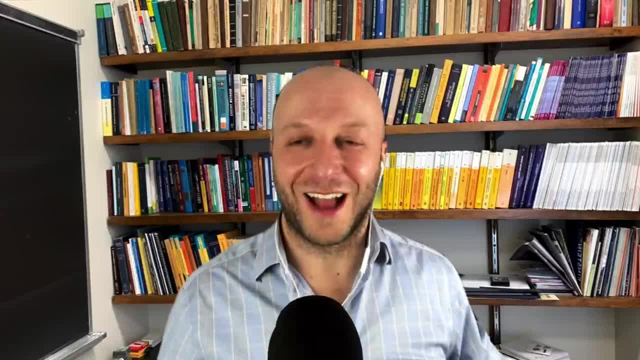 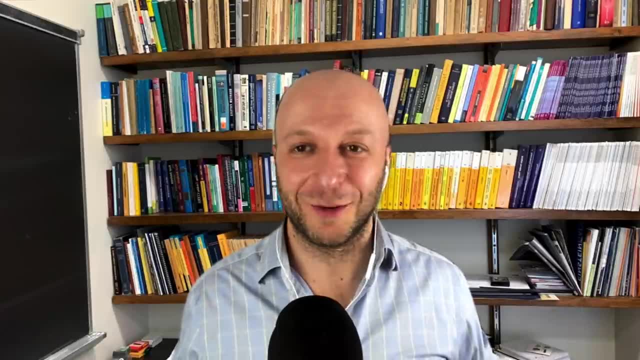 actually give you the value of 1 over 1 plus x. Right, and it might be nonsense. There's lots of math formulas that break completely when you do this. right. We have rules for a reason, but we should always know the extent to which the rules 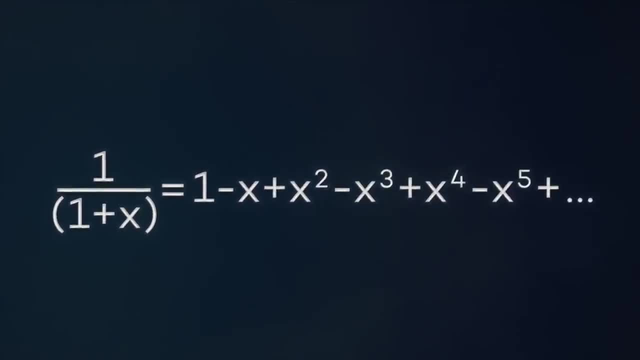 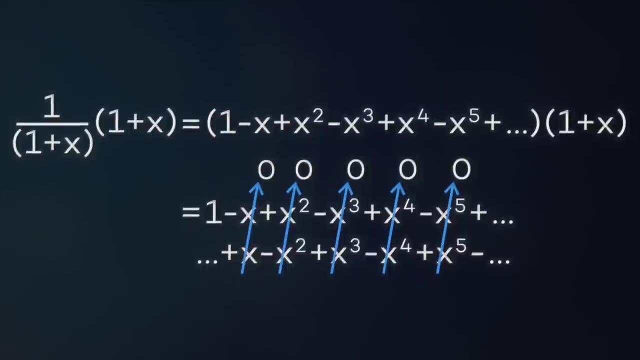 have a chance of working farther. If you take that whole series and you multiply it by 1 plus x and you multiply all that out, you'll see all the terms cancel except that leading one, And so that big series times 1 plus x is 1.. 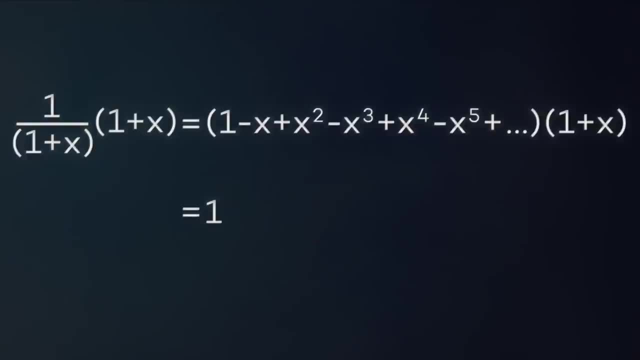 In other words, that big series is 1 over 1 plus x. That's how Newton justified to himself that it makes sense to apply the formula where it shouldn't be applicable. So Newton is convinced. the binomial theorem works even for negative values of n. 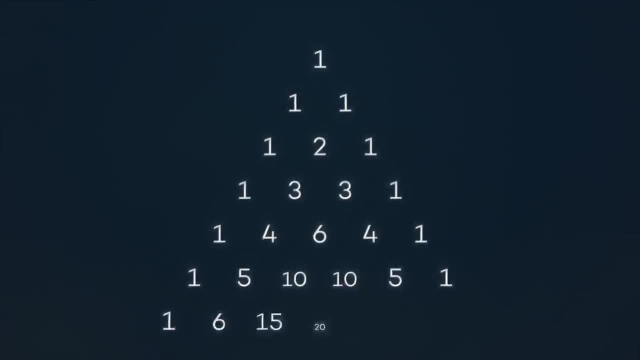 which means there's more to Pascal's triangle. Above the zeroth row you could add a 0 and a 1. that add to make that first 1.. And then that row would continue: minus 1,, plus 1,, minus 1, plus 1,. 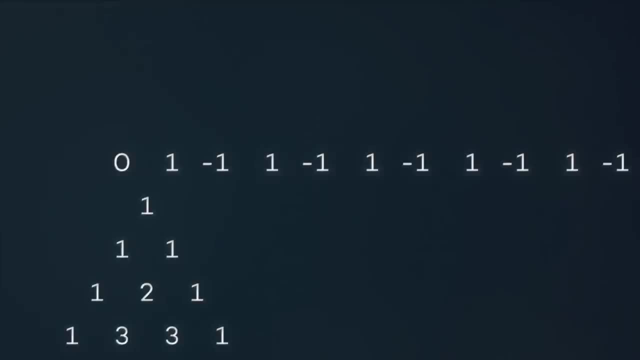 all the way out to infinity. And you know, outside the standard triangle the implied value everywhere is 0. And this fits with that. The alternating plus and minus 1s add to make 0 everywhere in the row beneath And you can extend the pattern for all negative integers. 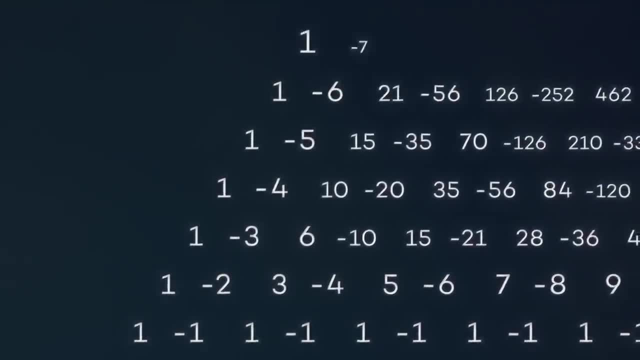 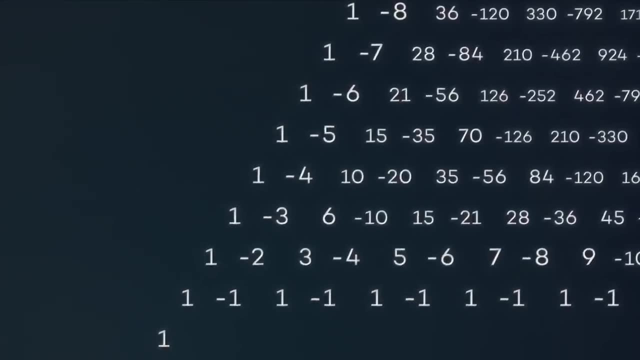 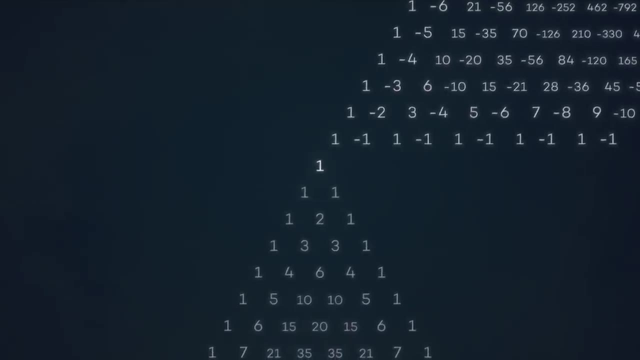 either using the binomial theorem or just looking at what numbers would add together to make the numbers underneath. And here's something amazing: If you ignore the negative signs for a minute, these are the exact same numbers, arranged in the same pattern as in the main triangle. 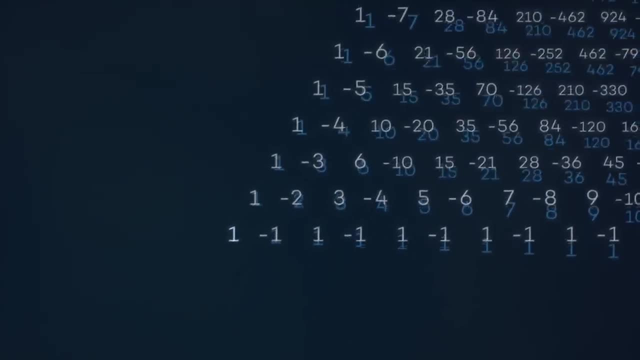 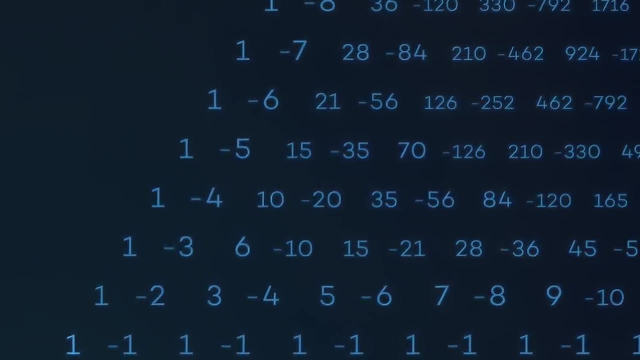 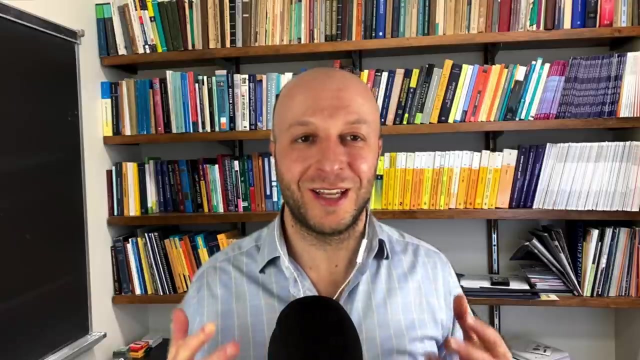 The whole thing has just been rotated on its side. But Newton doesn't stop with the integers. Next he tries fractional powers like 1 plus x to the half. So now, what does it mean? you take 1 plus x to the 1 half. 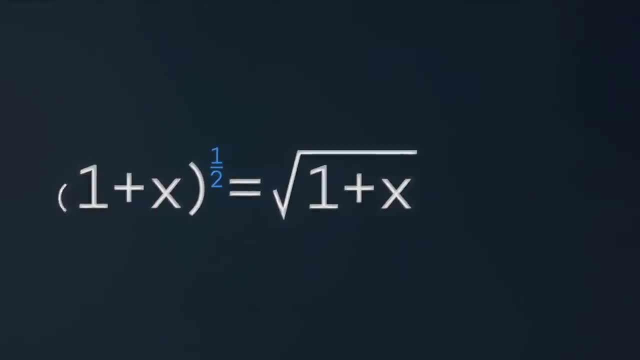 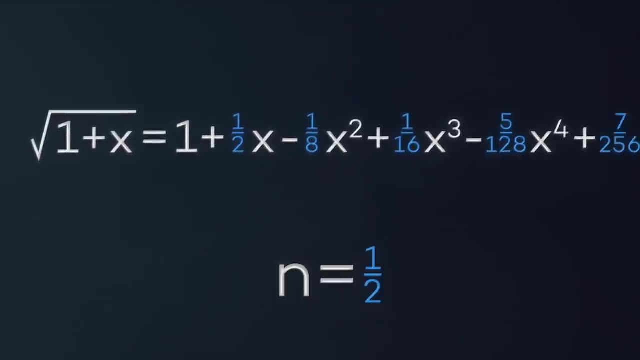 Well, that's the same thing as square root of 1 plus x, And he wants to understand. does that have the same expansion? Putting n equals a half into the binomial theorem, he gets an infinite series. That makes me think that we could actually. 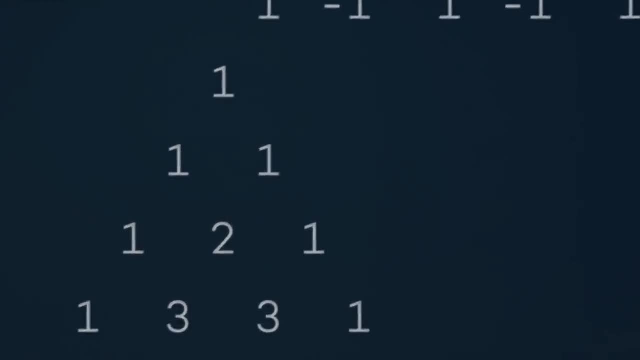 go into Pascal's triangle, blow it up and add fractions in between the rows that we're familiar with Exactly. There's even a continuum of Pascal's triangles Between 0 and 1, there's this, you know, a continuum of numbers that you could put in for powers. 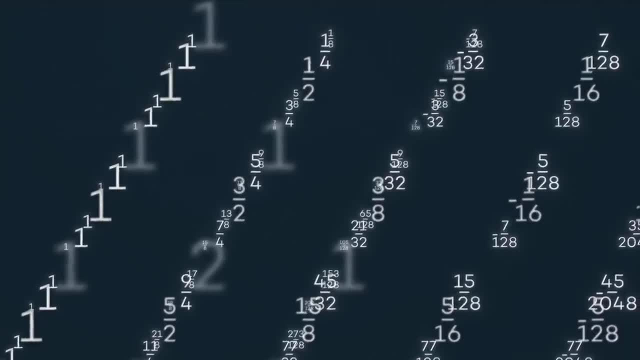 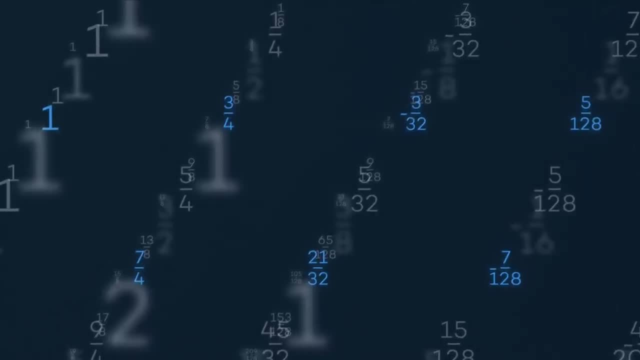 You can think of each fraction like a half, a quarter, a third, as existing in its own plane, where in each plane pairs of numbers add to make the number beneath them And doesn't have to be a positive integer anymore. 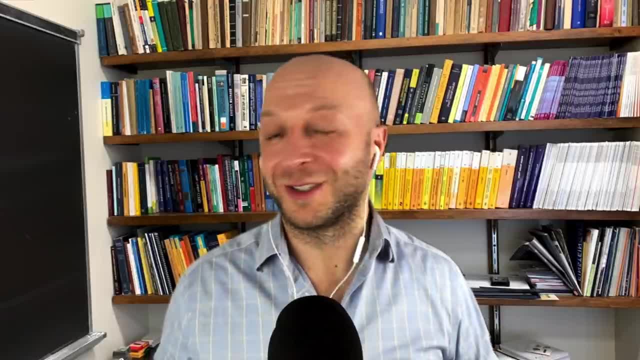 Doesn't have to be a positive integer, doesn't have to be a negative integer, doesn't have to be an integer. so now we're going to take n to be a half and he works this thing out, and then he could do all kinds of things. for example, he could work out the square root of 3. 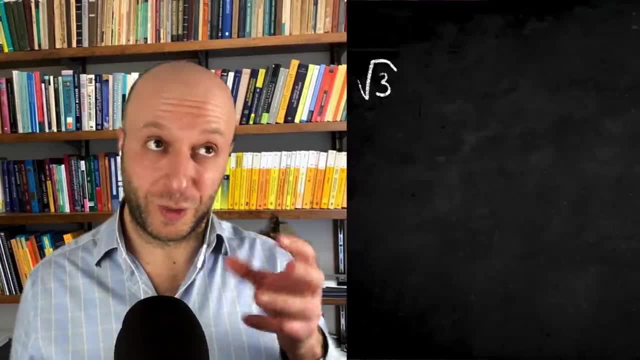 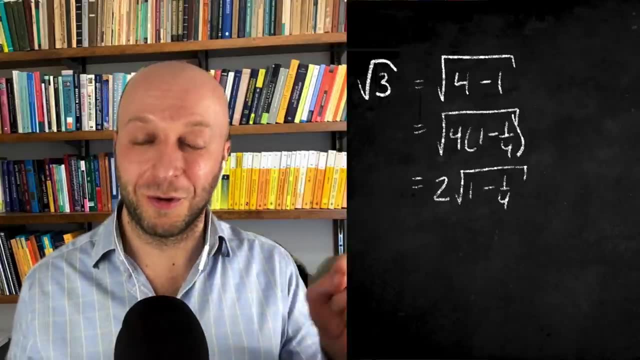 very quickly and efficiently, because the square root of 3- we can write 3- is 4 minus 1 and if we pull out a 4 then we get a square root of 4 which is just 2 times the square root of 1 minus a. 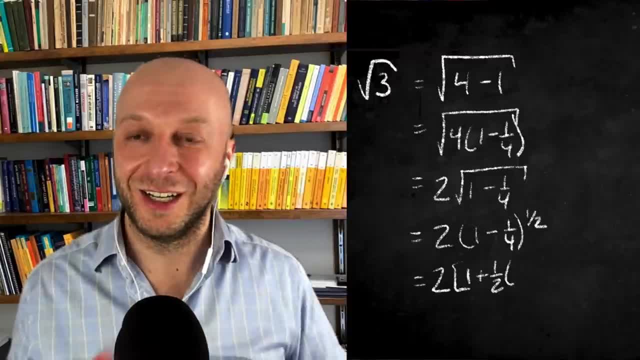 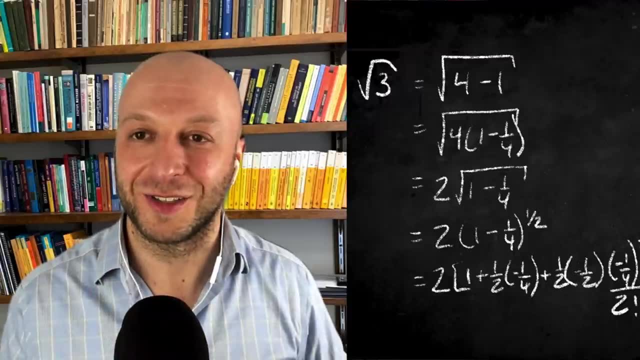 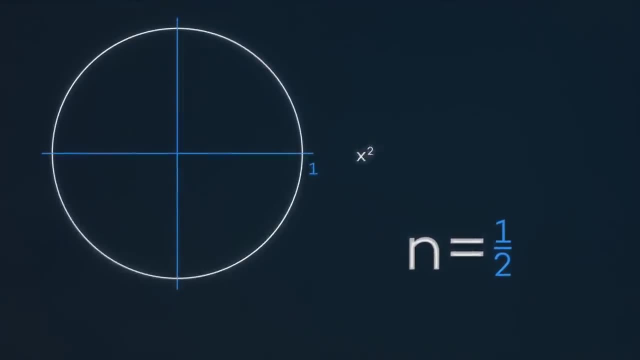 quarter. if you put in minus a quarter for x in this series, you'll get a very rapidly converging series expansion that will quickly give you square root of 3 to high accuracy. Now Newton is particularly interested in: n equals a half, because the equation for a unit circle is x. 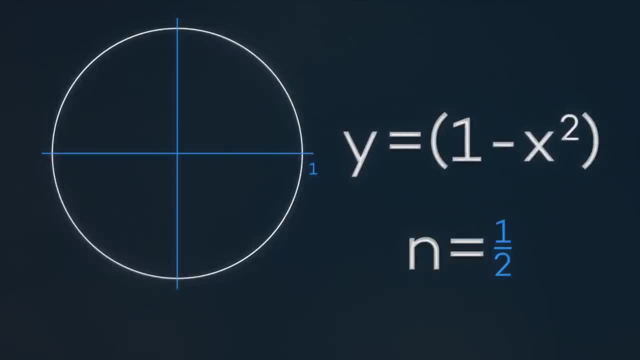 squared plus y squared equals 1, and if you solve for y, well, the top part of the circle is equal to 1 minus x squared to the half. This is basically the same expression he's been looking at. he just has to replace x by minus x squared. 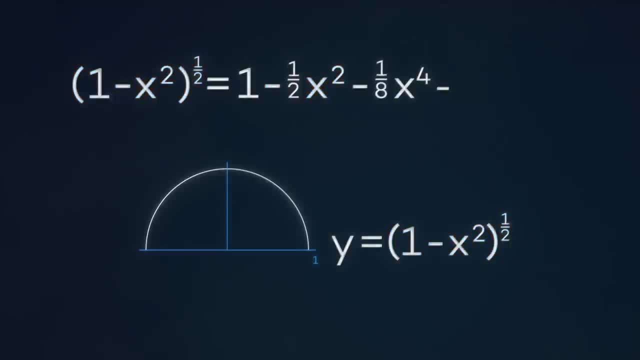 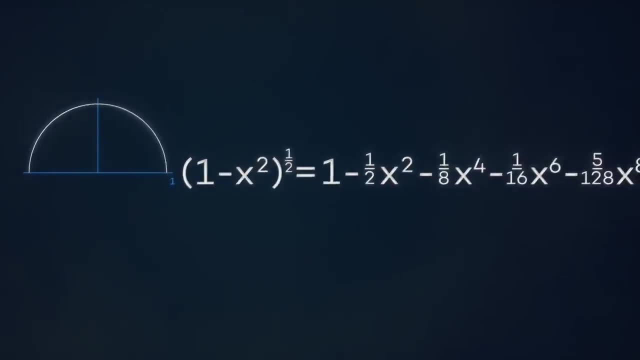 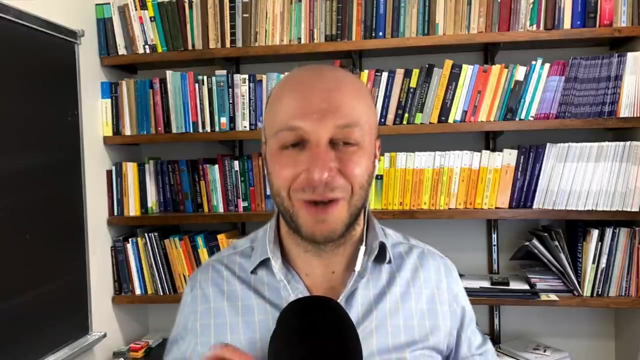 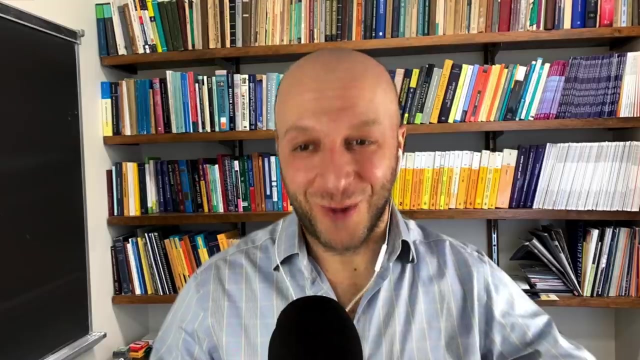 which adds in the square root of 3.. Now we have two different ways of representing the same thing, and whenever you have something like that, magic is about to happen. fireworks about that is about to go off. but how does he use this to calculate pi? Well, luckily for us, he had just invented calculus, or what he called the theory. 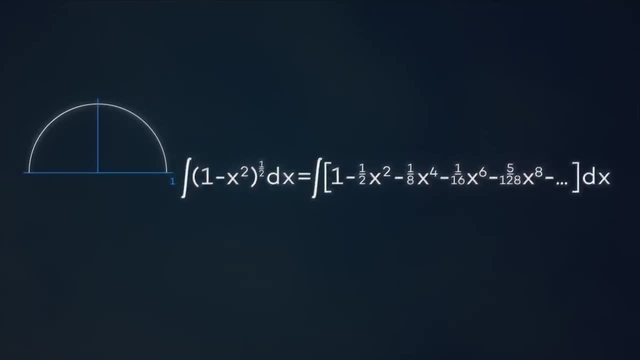 of fluxions. He realizes that if you insert a square root of 3 into the square root of 3, you integrate under that curve. as x goes from 0 to 1, you're getting the area under the curve which is a quarter circle. and he knows that the area of a unit circle is exactly pi r squared. 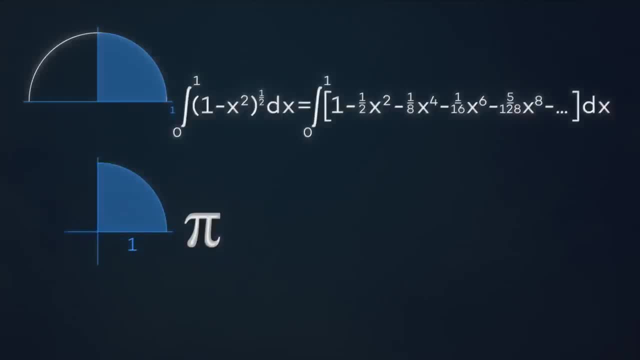 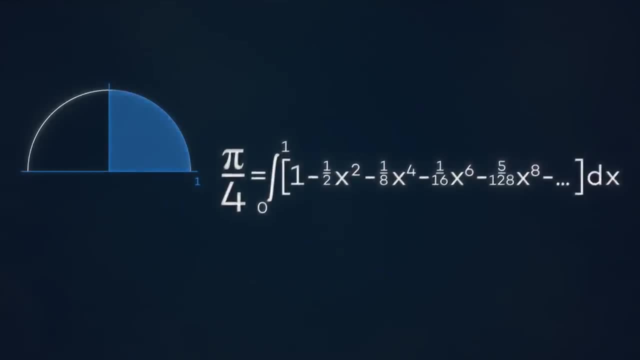 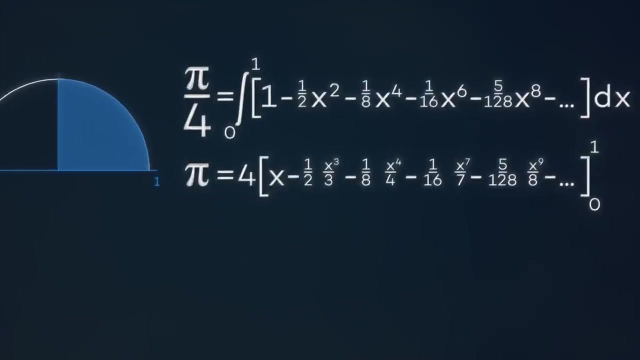 except r is 1, so the area is pi, and we want just a quarter, so the area is pi over 4.. On the other side he has this nice series and he knows how to integrate x to some power. You just increase each power of x by 1 and divide by the new power, and now you have an. 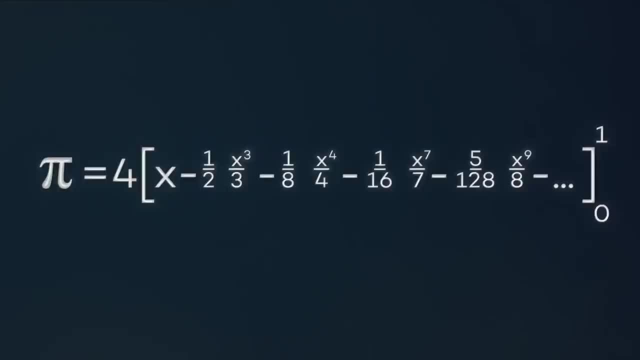 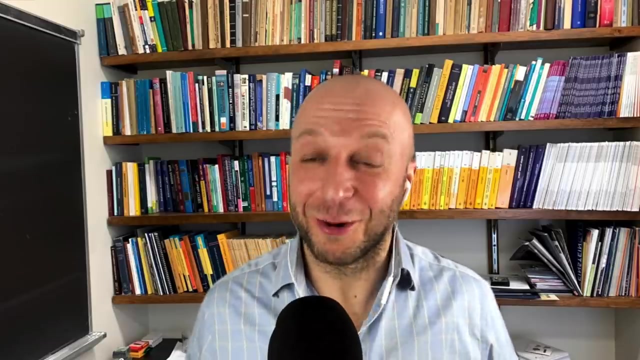 infinite series of terms which just involve simple arithmetic with fractions. You put in x equals 1 and you can calculate pi to an arbitrarily high precision. But Newton goes even further, adding one final tweak. A not good math paper has zero ideas. It's just pushing through things that everybody 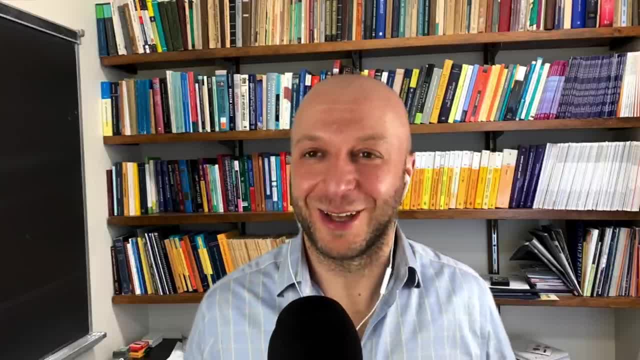 already knows but nobody bothered to do. Then there are good math papers that have like one new idea. that's like really shockingly new Newton's on new idea number 4 at this point, and he's about to have new idea number 4.. 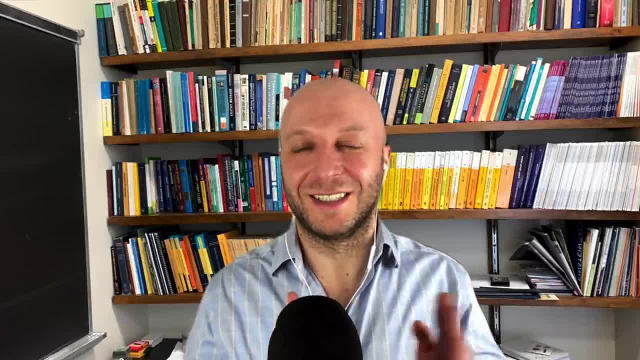 Newton's on new idea number 4 at this point and he's about to have new idea number 4.. A new idea, number 5, is, instead of integrating from 0 to 1, he's going to integrate just from 0 to a half. 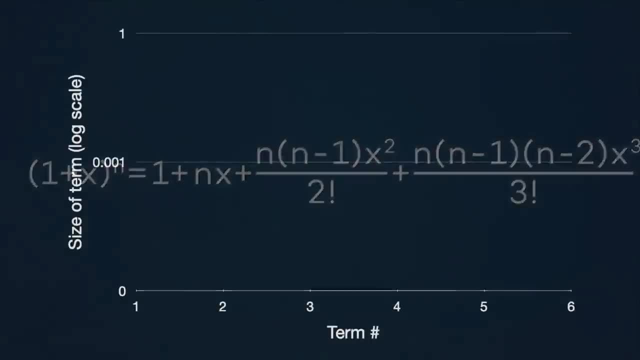 You know, when you have an infinite series you want the terms to decrease in size as fast as possible. That way you don't have to calculate as many of them to get a pretty good answer. And Newton sees: if he integrates not from 0 to 1 but from 0 to a half, then 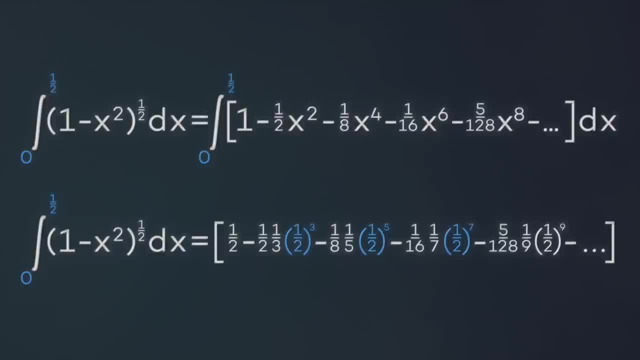 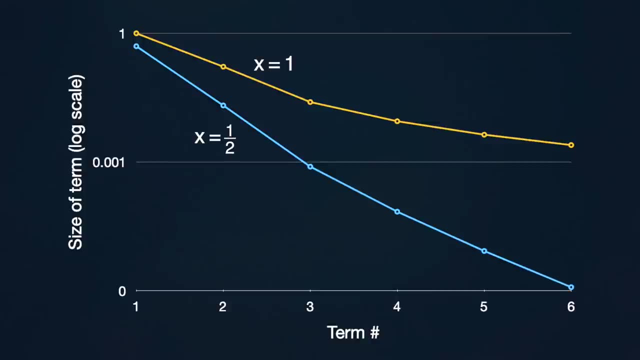 when he subs in a half for x, each term will shrink in size by an additional number. So if you integrate from 0 to 1, you get an additional factor of x squared, which in this case is a quarter. But if you only integrate to a half, what is the area under the curve that you're computing? 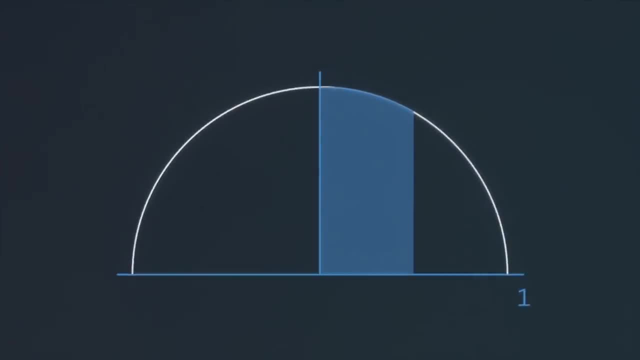 Well, it is this part of a circle which you can break into a 30 degree sector of the circle, which has an area of pi on 12, plus a right triangle with a base of a half and a height of root 3 on 2.. 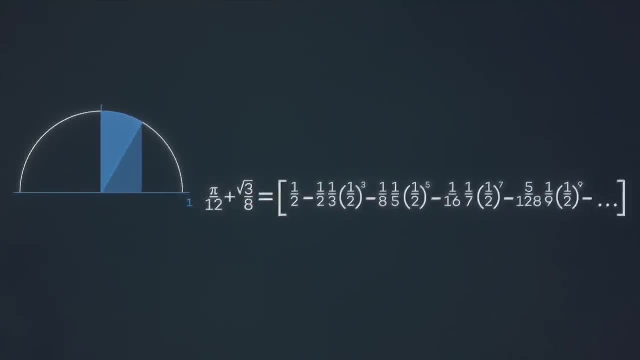 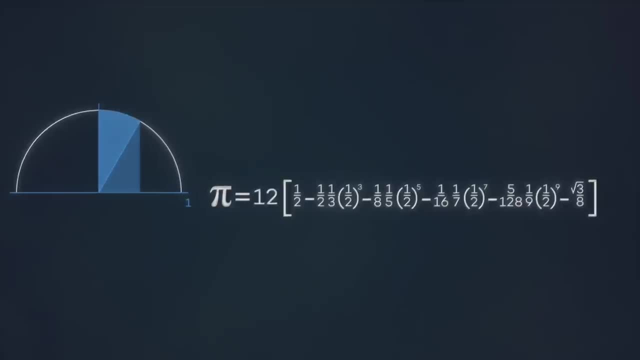 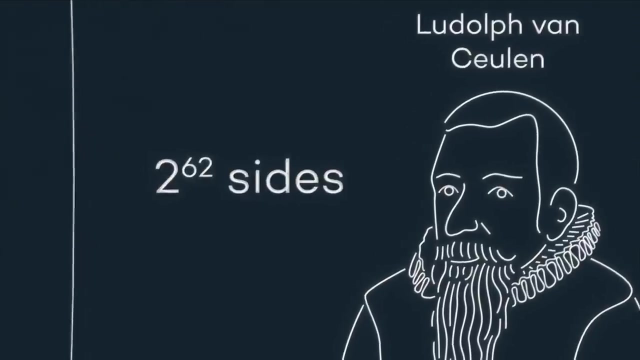 Now, if you evaluate only the first five terms, you get pi equals 3.14161.. That's off by just two parts in a hundred thousand, And to match the computational power of van Koehlen's four quintillion sided polygon you would only need to compute 50 terms in Newton's series. 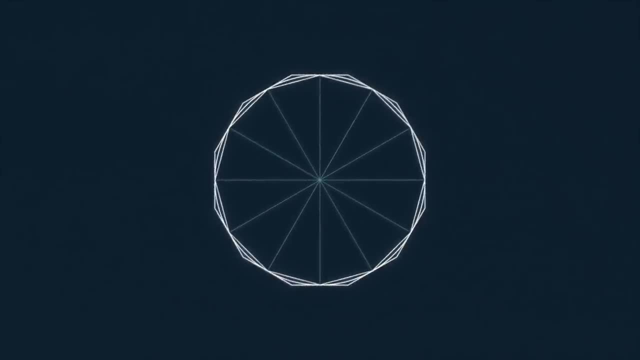 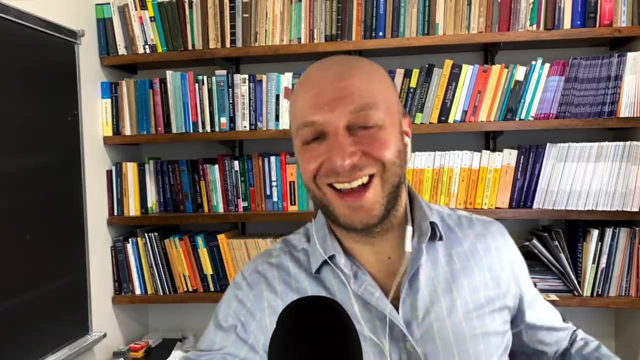 What before took years, now will take years. Now would take only days. So no one was bisecting polygons to find pi ever again. Why would you? Yeah, you do all that work and somebody comes along and beats you in a second. 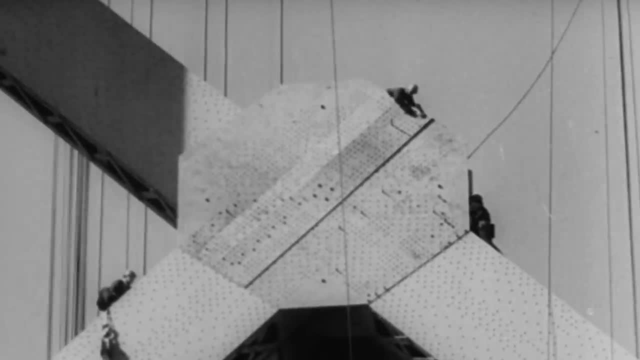 It's sort of like you know once someone builds a crane and then somebody else is still climbing up on a ladder to put a brick on a house like that's just not how you build houses anymore. We have new technology.